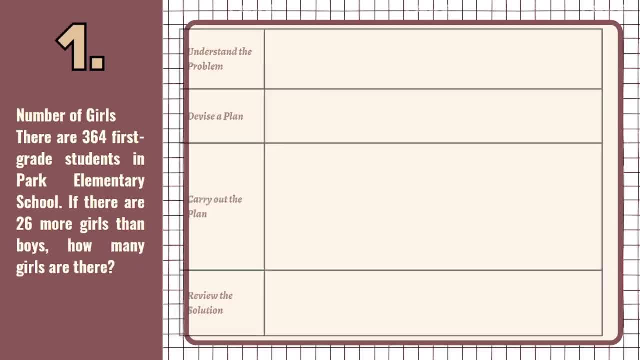 how many girls are there Applying the four steps of polyus problem solving strategy? the first one is we need to understand the problem. In this step we need to restate the problem in our own words, or much better if we translate it into Tagalog for us to easily. 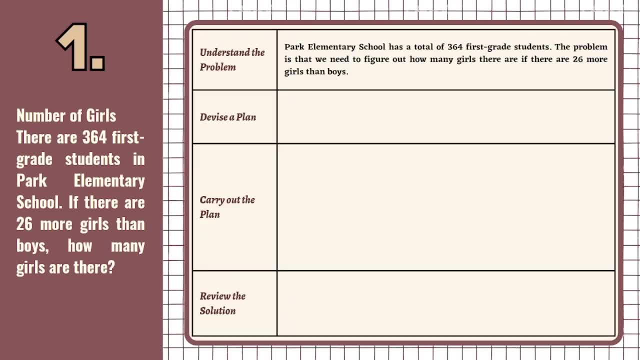 understand the problem. So Park Elementary School has a total of 364 first grade students in Park Elementary School. If there are 264 first grade students in Park Elementary School, the problem is that we need to figure out how many girls there are, if there are. 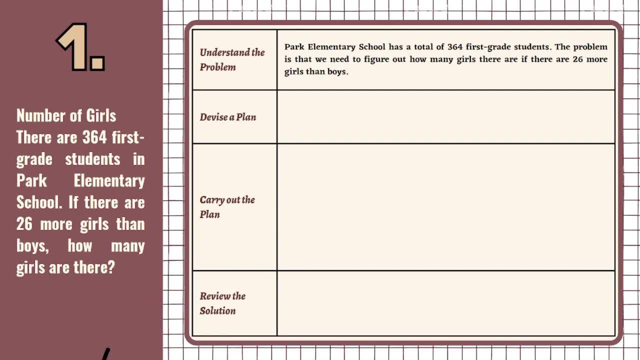 26, more girls than boys. The second step is we need to devise a plan. What appropriate strategy do you think we need to solve this kind of problem? So we will write an equation: If we represent the number of boys by b, then b is equals to boys and b plus 26. 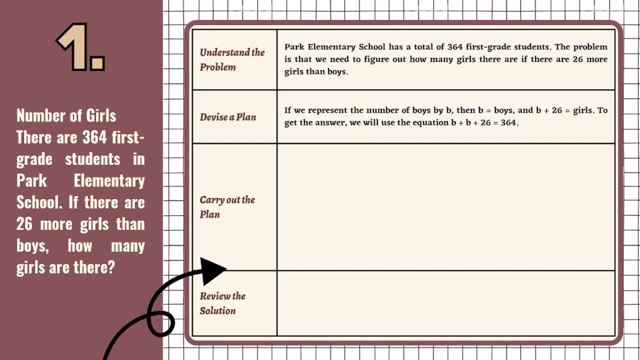 is equals to girls. To get the answer, we will use the equation b plus b plus 26 is equals to 364.. Carrying out the plan is the third stage. To begin write the equation b plus b plus 26 is equals to 364, which can be simplified to 2b plus 26 is equals to 364. 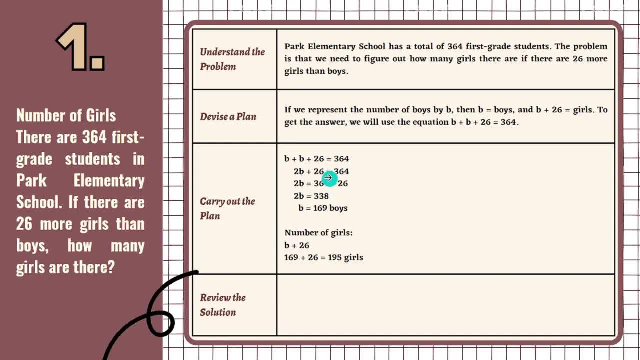 After that, substitute 26 on the right side and we'll make 2b is equals to 364 minus 26. And the answer for dot is 338.. Lastly, divide both sides by 2. The answer would be 169.. 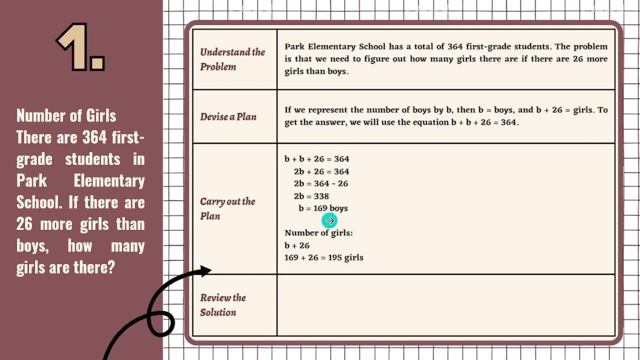 Therefore, the number of boys is 169.. Next, we must determine the number of girls using the formula B plus 26, which will give us: 169 plus 26 equals 195 girls. since RB is equals to 169, the last step is to review the solution since B.